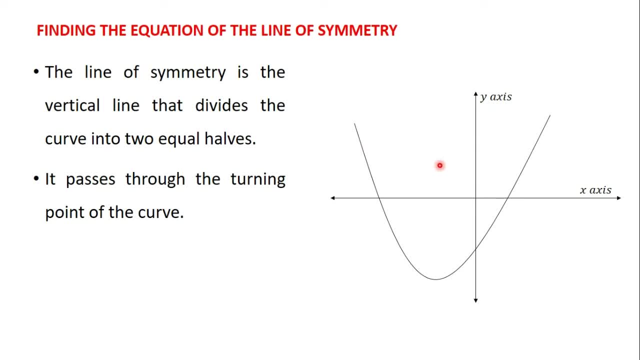 x-axis and the y-axis here, and this is the curve. The point here is telling us that the line of symmetry is the vertical line that divides the curve into two halves. So the vertical line that divides this curve into two halves is what is called the line of symmetry, the line 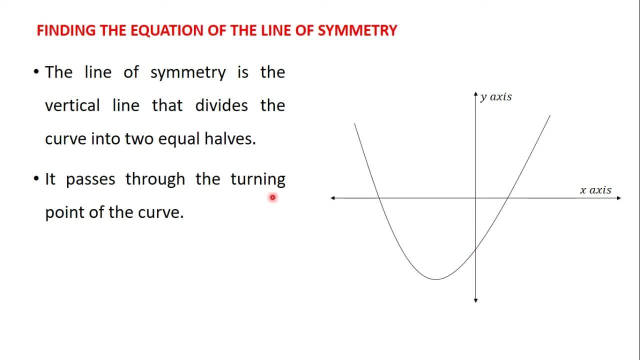 that divides the curve into two halves and it passes through the turning point of the curve. So let's say that on this curve, this is the turning point. The vertical line that passes through the turning point, thus dividing the curve into two halves, is known as the line of symmetry. util Если您--". 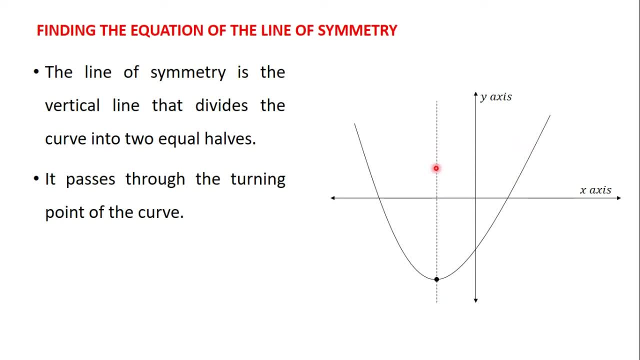 symmetry. so on this graph sheet, this is the line of symmetry, the vertical line that passes through the turning point dividing the curve into two halves. how do we find the equation of this line of symmetry? as we can see here, the line of symmetry passes through the turning point. so at the point where the line of 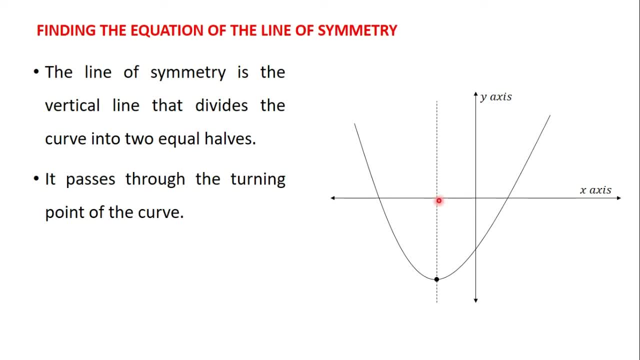 symmetry meets the x-axis, we will have the s coordinate of the turning point. so at this point, that is the point where the line of symmetry means x as this, you have the s coordinate of the turning point. let's say that that point is a. the equation of this line of symmetry is: x is equal to a. so to find the equation of 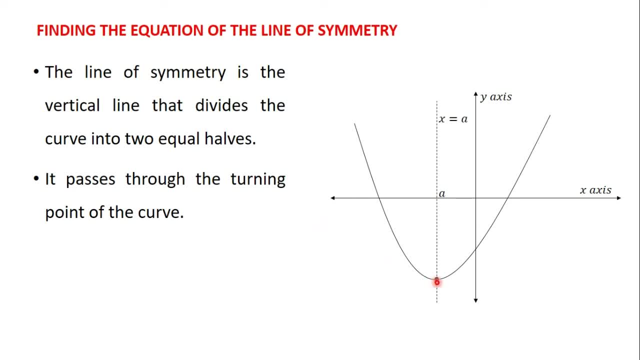 the line of symmetry. the first thing you need to do is to locate the turning point. then you draw a vertical line through the turning point. that vertical line will divide the curve into two halves. that line is known as the line of symmetry. to find the equation of the line of symmetry, locate the point where. 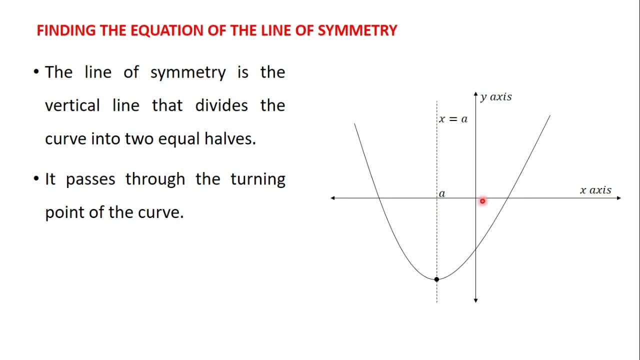 the line of symmetry meets the x-axis. on this graph, the line of symmetry meets the x-axis at point a. the equation of this line of symmetry is: x is equal to a. so I'll go right once again to find the equation of the line of symmetry. you locate the turning point and you draw a vertical line to: